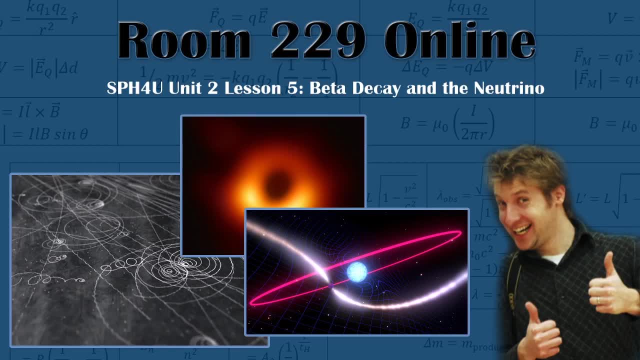 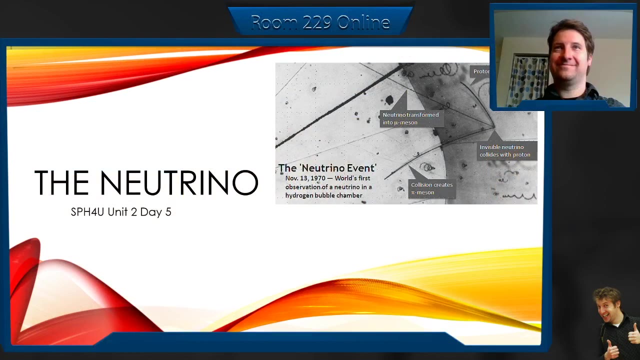 Hello everybody. so hopefully you guys have had a chance to look at all the elastic and inelastic problems that we did and if you had any troubles with those, put all the solutions on our website. If you have any questions, just send it to the Discord or send me an email. if 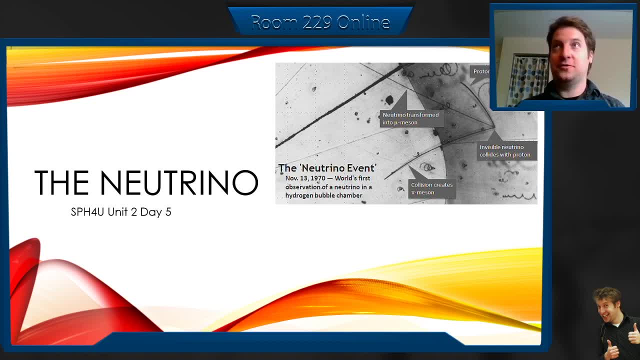 you'd like Go from there Now today. this is fun. okay, This is like a Mr Stone lesson. This is going to be fun. We're not going to divert away from, just, you know, the simple Newtonian kinematics and dynamics. here We're going to do some modern physics. 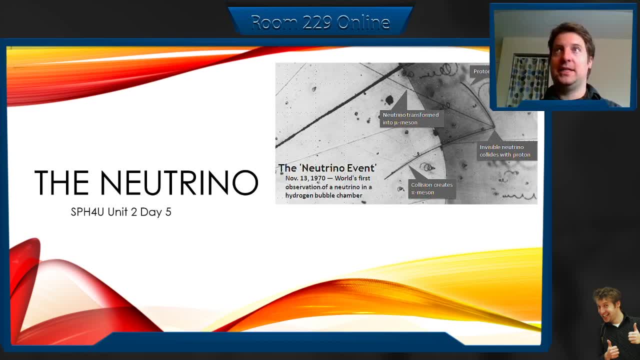 We're going to talk about some stuff that's actually happening now, some neutrino physics, looking at some real modern physics problems. okay, So we're going to talk about beta decay, which we- hopefully you guys have, I think I talked about in class a little bit. 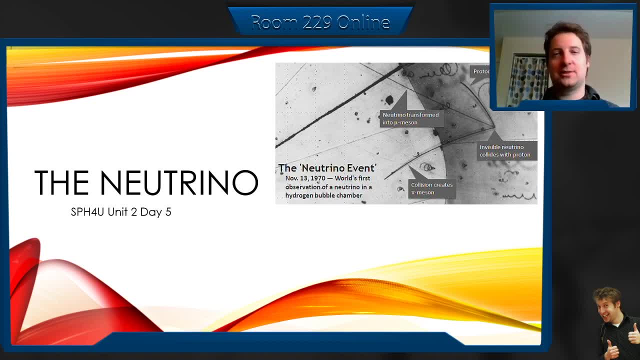 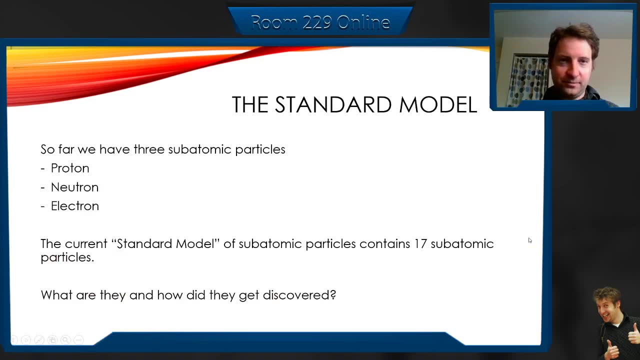 where electrons come from and that sort of stuff and weak interactions and all that sort of weird thing. So let's go, let's think about some of the stuff that we've done here. So let's start with what we know so far about the universe. what makes up all the stuff in the 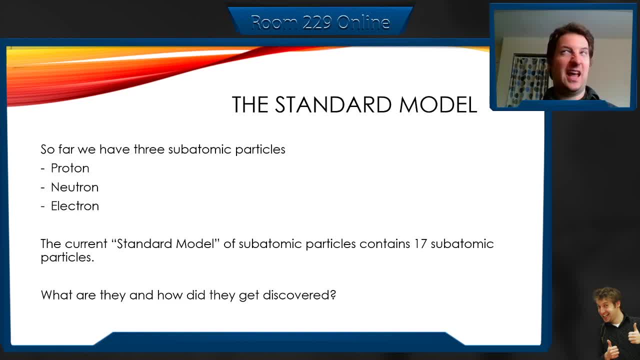 universe. So so far, according to you know, grade 10, even grade 11 chemistry, probably even grade 12 chemistry- there's only three things that make up the universe. We have protons, neutrons and electrons. You stick them together, you get an atom. 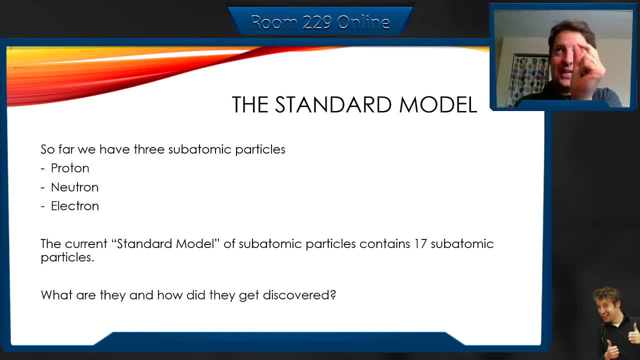 you do things, you do chemistry with those atoms. right, We have this little, tiny little grain of here in the middle of the thing. right, If this whole room was an atom, there'd be this tiny little speck of sand that contains all the mass, and they call it the nucleus, and it contains all. 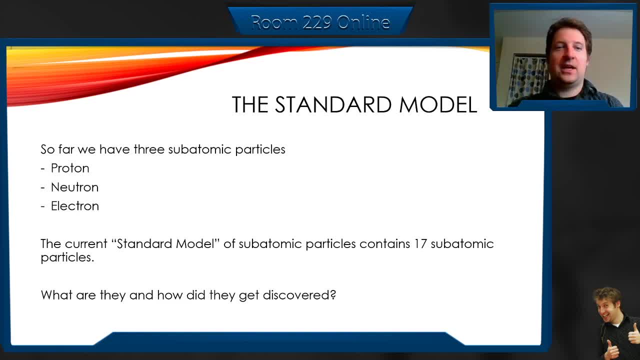 the protons and neutrons, the nucleons we can call them, And around them is this haze of electrons buzzing around in these shells, these S and P and all D orbitals and all sort of weird stuff like that. right Now, that's what you guys have learned. The modern view of the universe is: 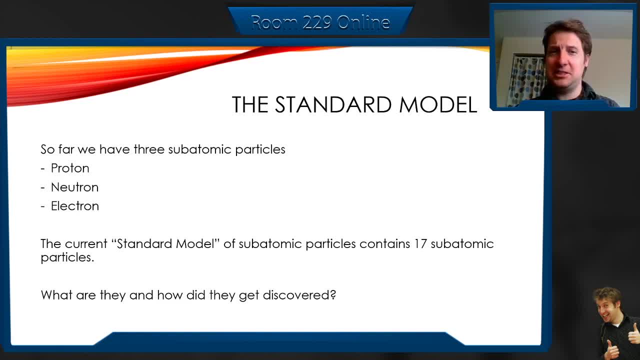 a little bit more complicated than the modern view of the universe. but it's a little bit more complicated, It's not much, it's just a little bit deeper into those nucleons and there's a few extra things. But we call this the standard model of subatomic particle physics. It's called 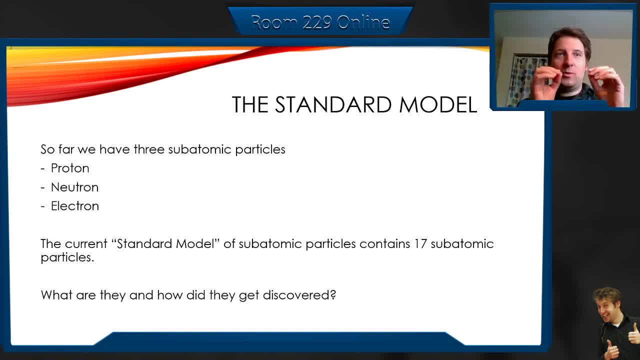 particle physics, the idea of all this, this idea of what is the universe made of and how do all those things that make it up interact with each other? And currently there's 16, and then one extra, so 17 subatomic particles. What are they? How did they get discovered? 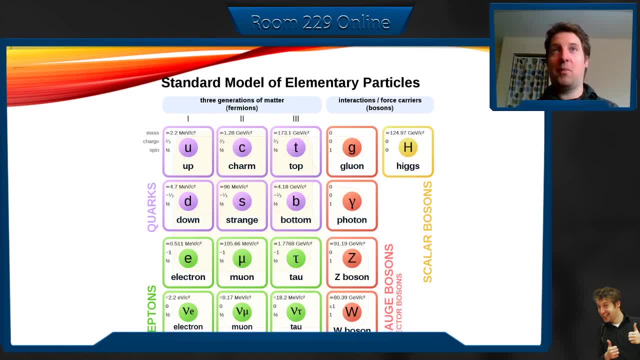 This is the picture that we see now of our modern view of the universe. So we have. what do we have here? Where's my pen? Maybe with my little? where'd it go? Where are my funky little? there it is. 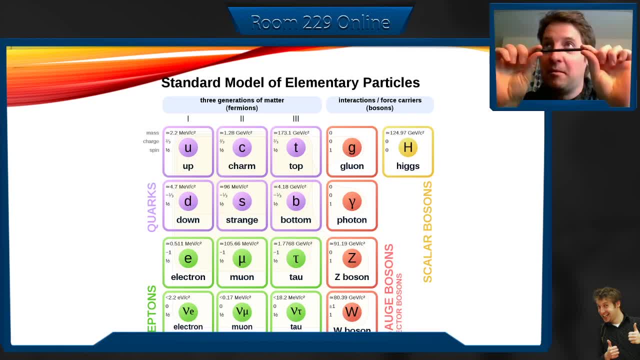 found it A little computer pen kind of fun to play with. Okay, so here we have what we call the quarks. So this group here, you can't even see the cursor. Yeah, yeah, This group, this is the quarks. 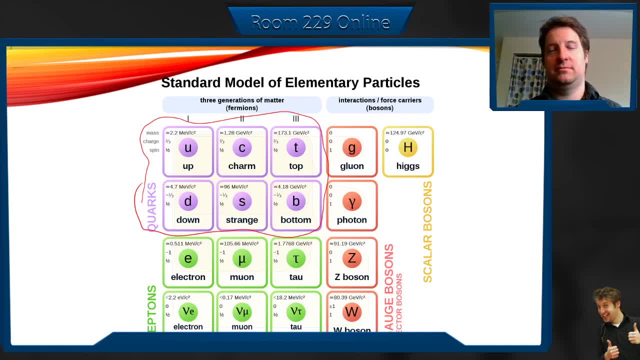 this is what makes up all the mass in the universe, What we interpret as mass. okay, So we've got up down which makes up most of our protons and neutrons, charm, strange bottom and top. okay. 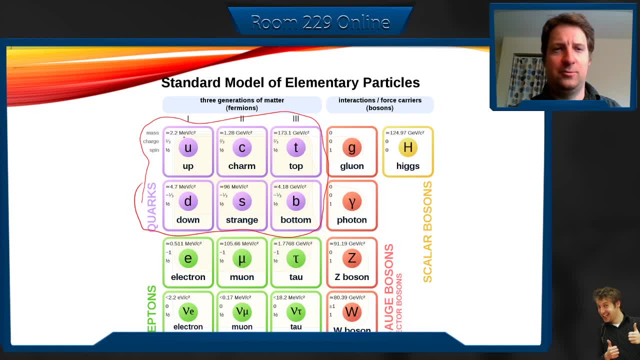 And it shows here. they have sort of effective masses in this really strange unit: mega electron volts per e squared, which we'll talk about this in unit five. okay, So this is the mass of the quarks, And then we have much smaller things. We have an electron. We all know what electrons are. 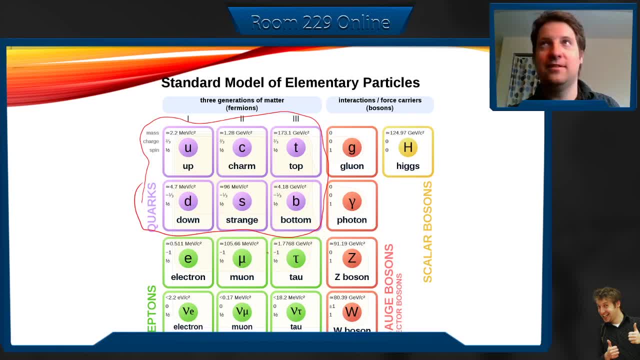 Then we have a slightly different flavor of electron fermionic flavor. These are called the leptons. All this whole left-hand side- here you can break this up: We got on this side. these are the fermions And these over on this side are the bosons. 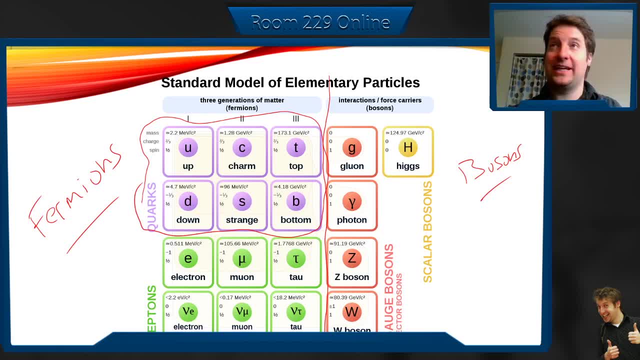 And the difference is that fermions can exist- I'm sorry, can't exist- in the same quantum state They have. you can see here, they all have spin halves. These all have half spins, Every single one of these. yeah, they all have half spins, which means that they obey what we call Fermi. 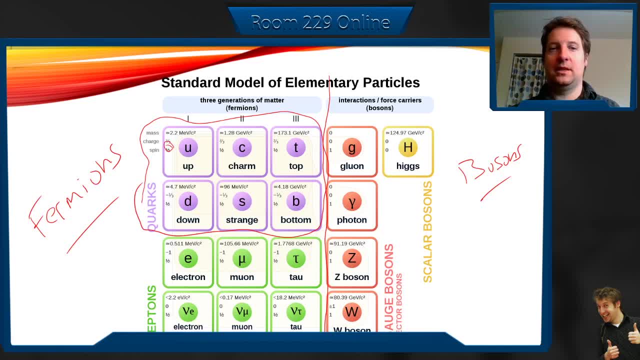 statistics. They can't exist in quantum state, Like, for example, when you looked at your in grade 11 chemistry. we have remember we had to do Pauli's question right. We had to do Pauli's exclusion principle. You had to put electrons up and down, But in that quantum state there can. 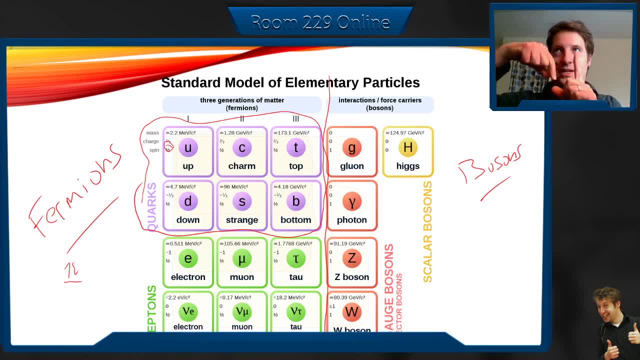 only exist an electron up and an electron down. Bosons are different because they can all they can coexist in the same sort of quantum state. So photons don't care about the fact that they're together. They all can have the same quantum state. One thing we can actually take: we can 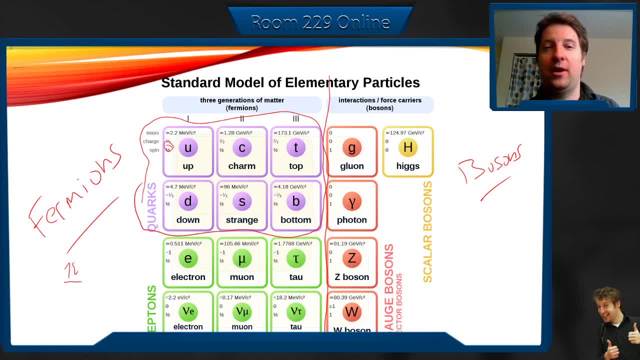 take matter, and if you get it cold enough they can sort of pair up with each other. They can end up behaving like bosons. You can take helium and the helium atoms can get into a state when they're cold enough, where they have integer spin. Then the 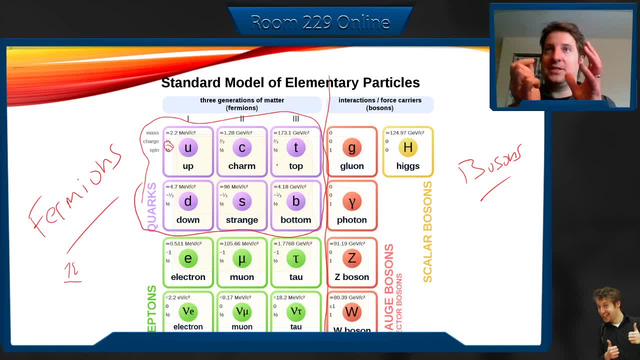 whole helium mass can all end up with the exact same quantum state. We call this a Bose-Einstein condensate. This is where you get superfluid helium, where every single atom, all the atoms, all 10 to the 24 atoms of helium in this container of helium, all are in the exact same quantum state. 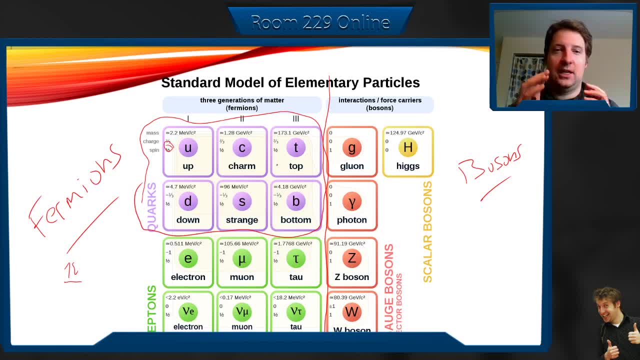 And they behave like a superfluid. They have superconductivity. Electrons can pass through them with no resistance. They have no viscosity. They can come out of the thing. It's very strange. Only happens at like, I think, for helium. it happens at negative 2.7. 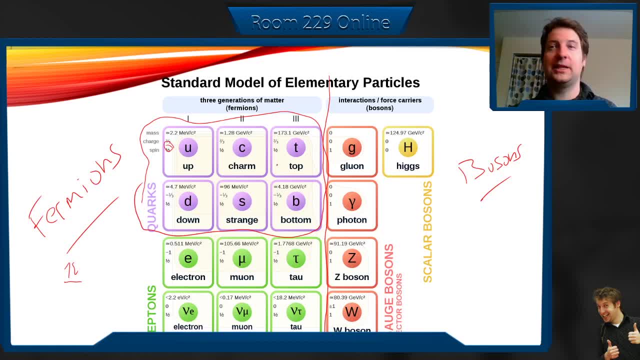 Kelvin, I think It's very, very, very cold, But liquid helium- look it up, Fun stuff. Okay, So there's the fermions on one side, bosons on the other side. Okay, So we have all the matter. 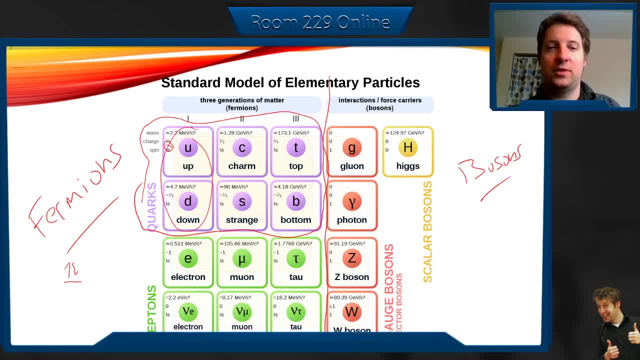 our nucleons, mostly up and down. That makes our protons and neutrons. Then we have our electrons that we're used to extra flavors. Then we've got these funky things called neutrinos that are completely strange. Notice, here we don't have a mass, We have a less than We don't know what. 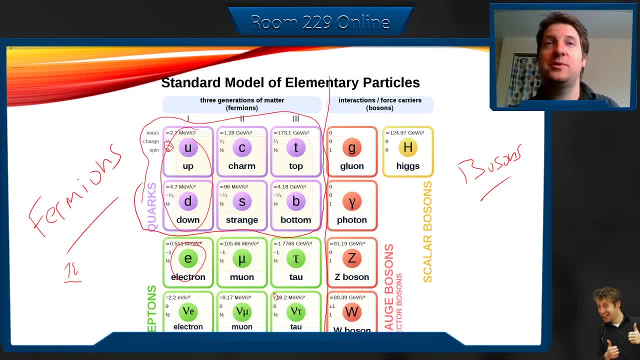 the masses are of neutrinos. We're still working on that. That's one of the undiscovered things. We have an undiscovered thing called neutrinos. We have an undiscovered thing called neutrinos. We have an upper bound here for the mass right. Sorry, So it has to be less than So. yeah, it's an upper. 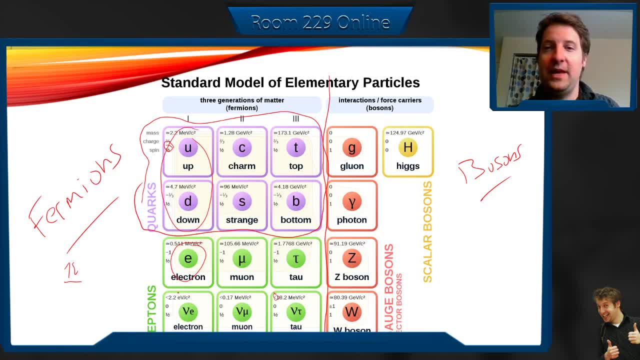 bound of what our masses could be. Then we have over here, we have the bosons. These are the force carriers. We call them force carriers because they are able to pass on our forces, our four elementary forces. Well, gravitons aren't even in here. 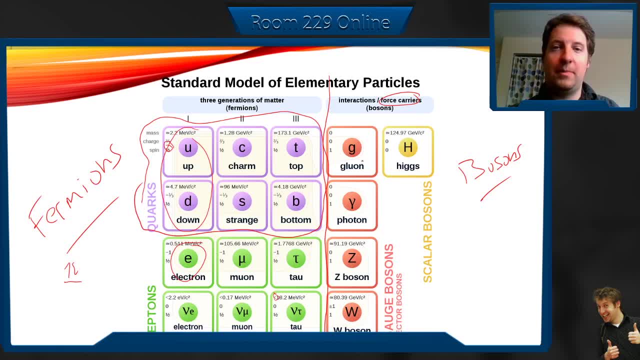 We have gluons that obey the sorry, that pass on strong nuclear force, Photons that pass on the electromagnetic force, And these two, the Z and the W bosons- sorry, the Z. you can call this a Z, not Z zero- And this is a W plus or minus. These are the weak interaction force carriers And 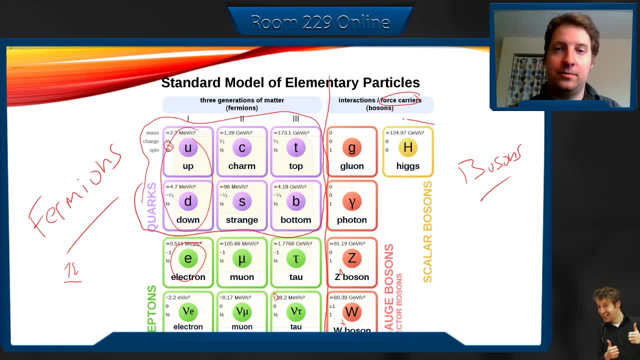 there's a neutral one and a charged one, And then we got this really fun. This is very new. This is as of 2007, when we started to use what we call the Large Hadron Collider. I think is it 2007? Maybe it's not Get rid of that. I. 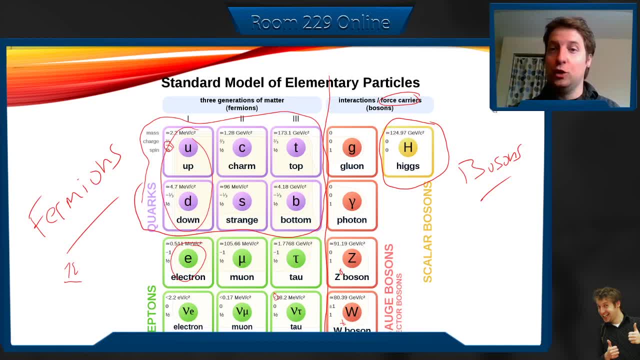 don't remember exactly here, But we just discovered a new particle called the Higgs boson that transmits what we call the Higgs field, And we think this is where mass comes from, This is where inertia comes from. That last fundamental problem that we're going to talk about is the Higgs field. 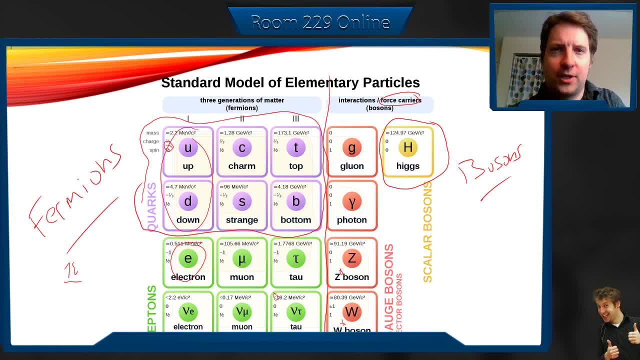 The problem of physics, of Newton's first law: everything that has mass has inertia. Why? And we think it has to do with the Higgs boson. So this is our view, This is the particle physics view of the universe as it is. These are the 17 things that make up everything. This is our view of how. 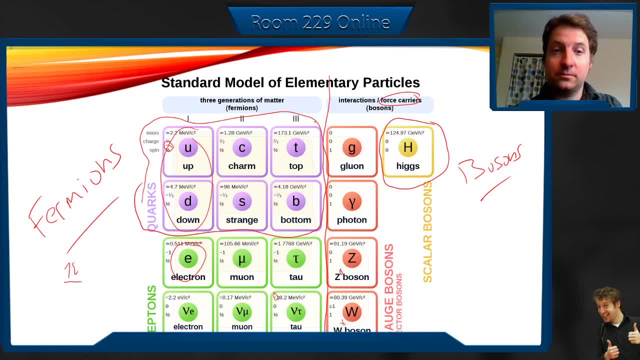 the universe is made. We have quarks, We have leptons- Altogether we call fermions. Then we have bosons that pass on interactions. So these are the types of matter. So you have matter in the form of quarks, electrons and neutrinos. Then we have force carriers, which we call bosons. 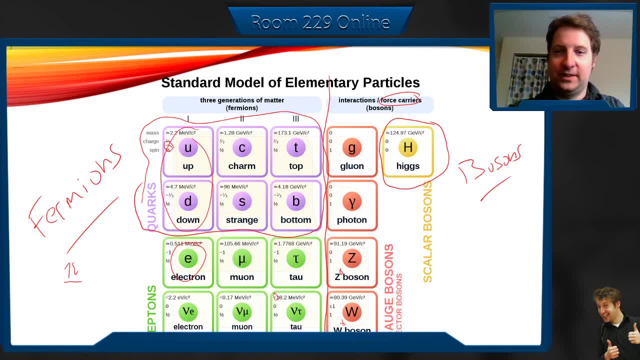 And don't worry about the fact that there's a vector and scalar, but a gauge boson- This is one of the favorite words for modern particle physicists- Gauge fields. If you look at the interaction of gauge fields and quantum chromodynamics, all that sort of fun stuff. 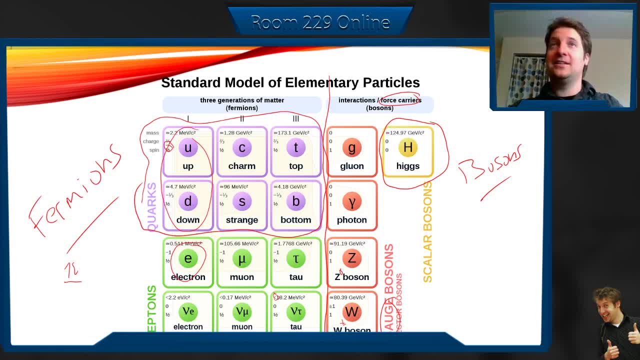 So this is the universe. You are looking at the universe as we know it now. Remember that anytime we do physics, it's always an approximate view of the universe. Newton was not wrong. He was right to a certain accuracy, a certain precision. Then we start looking closer and we 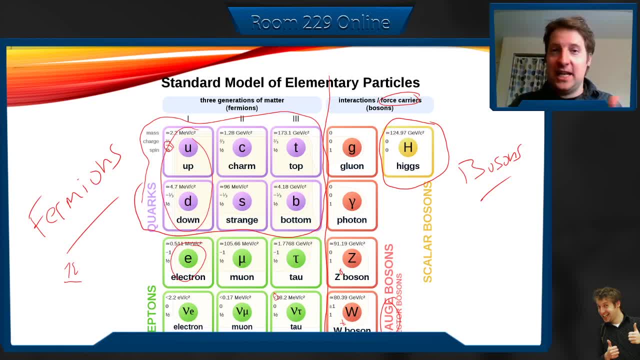 find little mistakes and we refine the picture. It's not saying that anything is wrong. It's not saying that anything was wrong before this. Your view from grade 10 of an atom is, let's say, sodium 12p- sorry, 11p, 12n. then we do this: 4 rather for diagram right, 1, 7,, 8,, 10, and 11.. 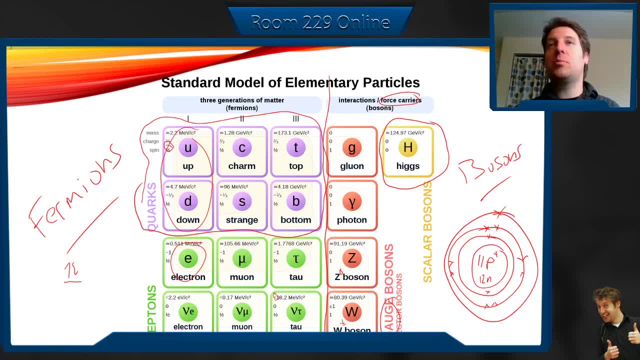 That view of a sodium ion atom, sorry, is not wrong. It's just an approximation of the truth. It's not saying that that is false, It is an approximation. And we learned all about those other things like orbitals and that sort of stuff and go on from there, But this is our most. 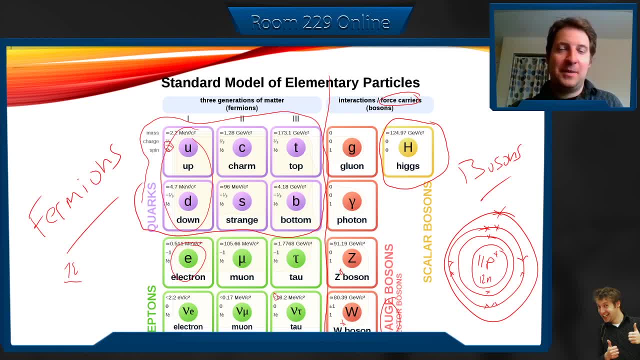 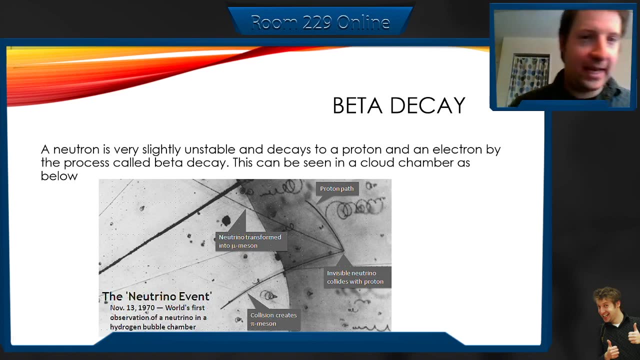 accurate. It might be wrong, It might be like there might be something fundamentally wrong with this and we have to refine it, But this is as of 2020, this is the most accurate view of what the universe has made out of Okay. So let's talk about beta decay. So beta decay ends up being 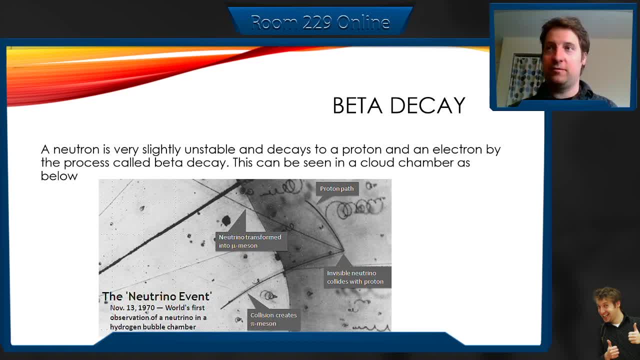 how we. it's one of the ways in which things fall apart, Okay, One of the ways in which stuff decays. It's a nuclear process in which nucleons, or the nucleus of atoms, fall apart and give off stuff, In this case, electrons. So the first time that we've talked about this is from a neutron. 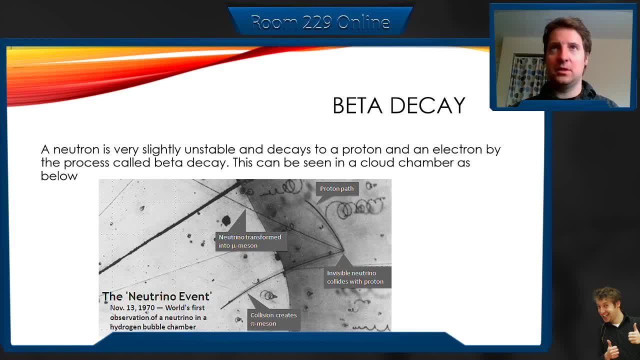 So neutrons are very, very slightly unstable. Neutrons can't actually exist for infinite time scale. Protons, we think, have an infinite time scale, but we have no idea. We don't know yet As of now. protons have an infinite time scale. 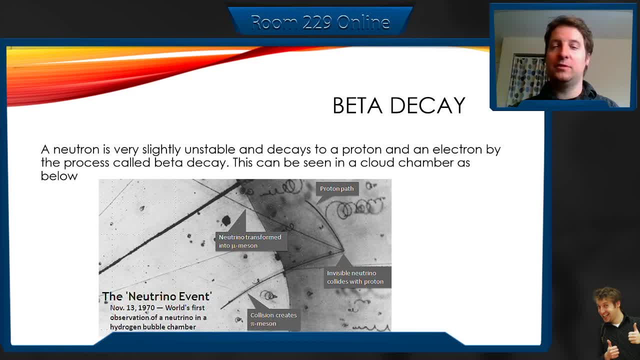 However, neutrons, we know, are slightly unstable and are able to fall apart. They decay into a new proton. So the neutron becomes a proton And while it does that, it gives off an electron. This is a process of beta decay And this, this is actually beta. 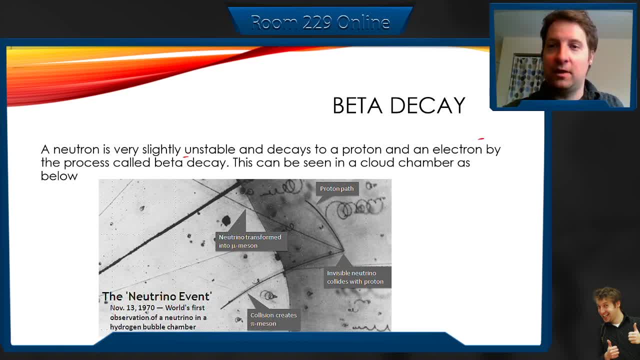 minus decay because it gives off a negative electron. right, There's actually beta positive decay, which is when we give off a positron, which is the antiparticle of an electron. So here this is actually shows us a an event in which a neutrino 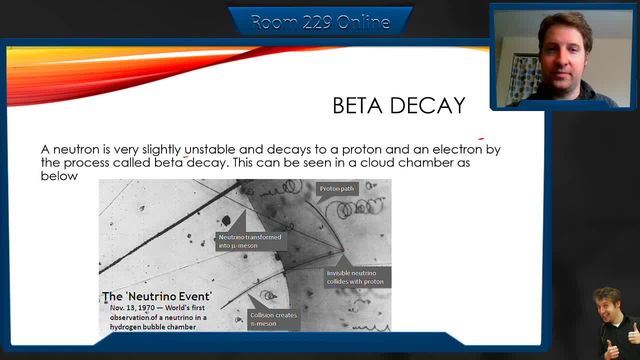 I'll talk about that later- comes along, So it comes along here and it hits a neutron. We can't see a neutron in this. This is called a neutron, So it's a neutron. So it's a neutron, So it's a neutron. 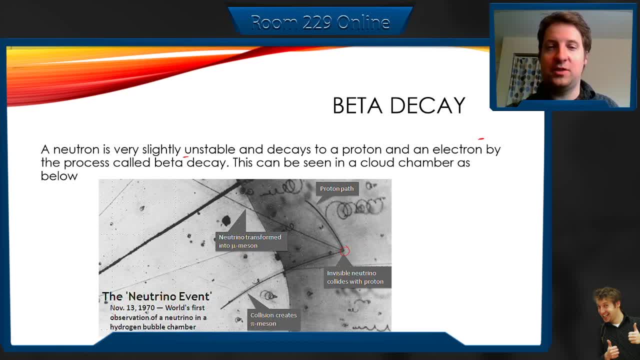 It's called a cloud chamber picture. This is, cloud chamber is a bunch of suspended alcohol And when charged particles whiz through it at high speed, it condenses on them. You can't actually see them here, But at this point a neutrino came along, hit a neutron and it broke. 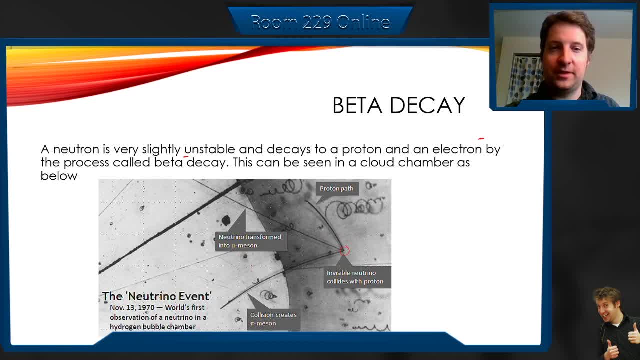 up into a proton and then a bunch of extra stuff here, So this is the first time that we actually saw this is a special type of of beta decay. They gave off a bunch of mesons. Mesons are two slightly different, But let's not worry about that for now. This is just showing a proton. 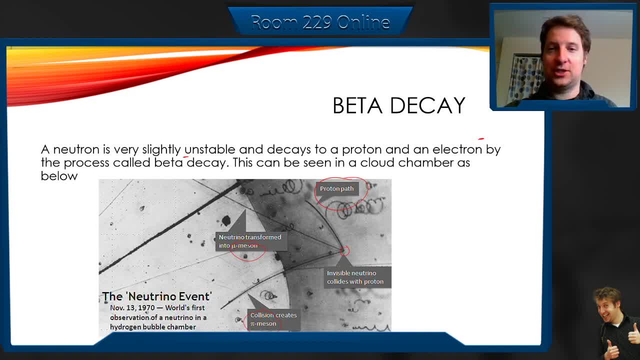 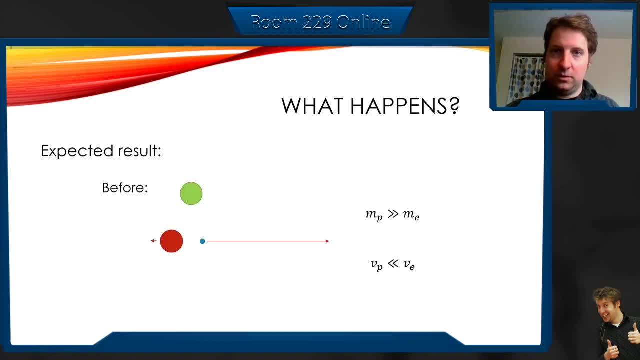 decaying from a, a neutron, And you can't actually see. It's invisible stuff. Hey, Oh, let's see what happened. So this was the view. of this is what we would see from a, a Newtonian viewpoint. Okay, so we have our all, this is our, our, our neutron here And it breaks. 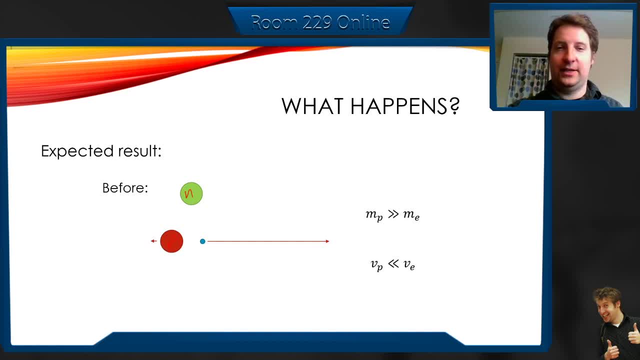 up into a proton and an electron. And notice, because the proton's mass is much, much, much higher than the electron's mass by a factor of 10 to the. what is it? 10 to the 10 to the, 4 times bigger, it's like 10,000 times heavier. 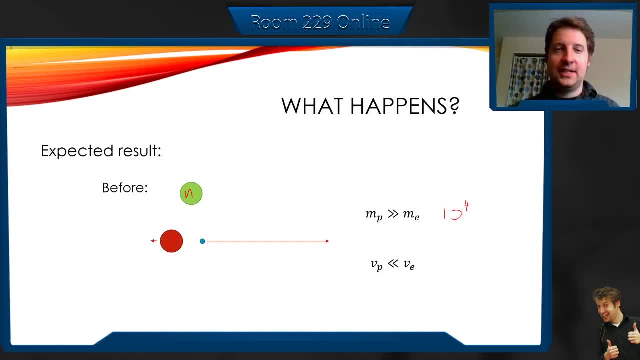 2,000 times heavier. So that means that the the order of 10 to the 4, which means that the velocities, because of conservation of momentum, the velocities are also going to be in that same order, 10 to the 4- times different. This electron's going to whiz away. 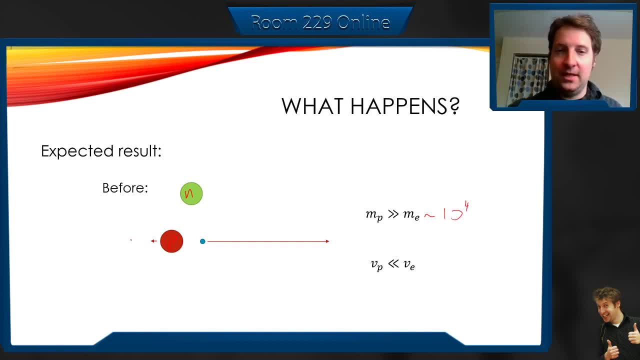 it's super fast and the proton's just going to cut it off. But the important thing is that this whole system is one dimensional. they're co-linear with each other. So what would we expect to happen when a proton and a neutron decay from a neutron? A proton and a neutron are made when that neutron 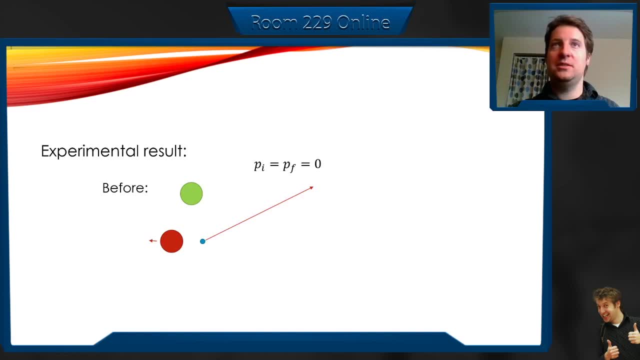 decays. However, what was actually seen was actually observed that the electron whizzes away. So, because we know that conservation of momentum has to be true, there has to be a invisible sort of particle that we can't at this point. we're talking about 1930s here. 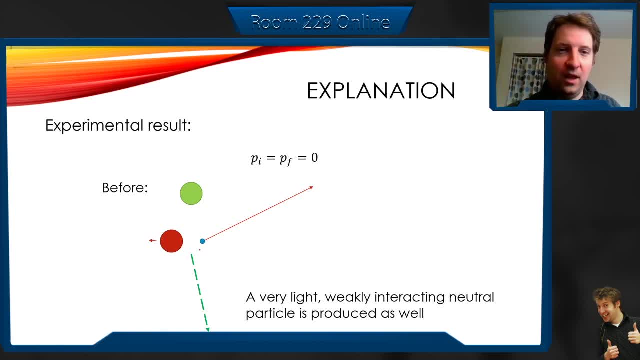 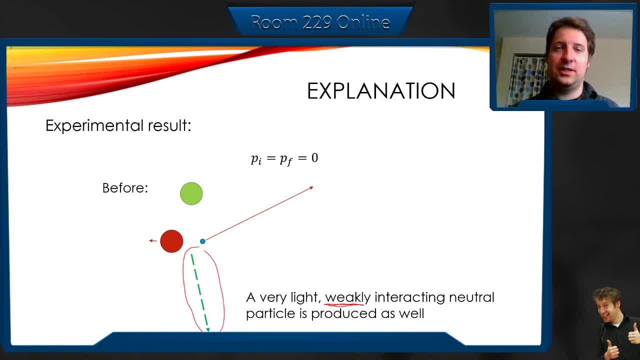 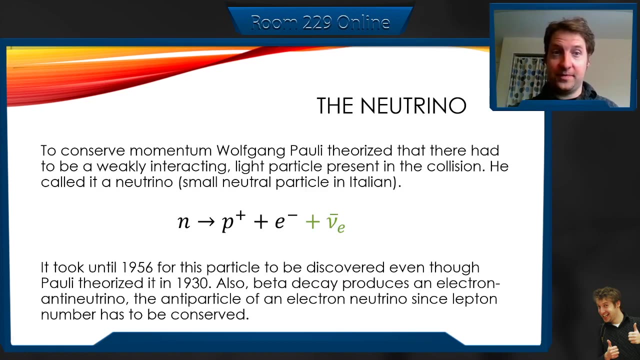 and it has to be produced there. So this is to satisfy this equation. if that was broken, then that's something fundamentally wrong with our understanding of physics. We want to keep that going, so we have to have this thing And to conserve this momentum, a guy called Wolfgang Pauli- again with the Pauli Exclusion. 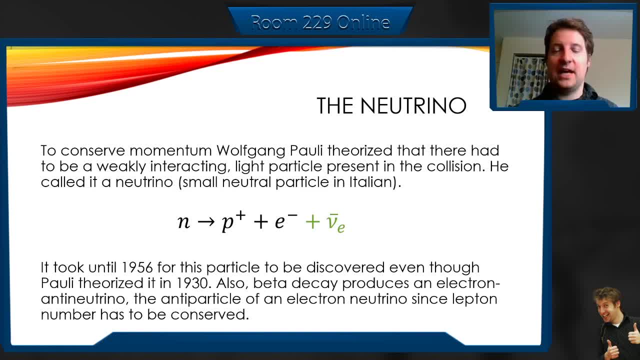 Principle, same guy. He came along and theorized that there has to be this third thing showing up. A third guy showing up. it's a weakly interacting light particle that has to be present in the collision. He called it a neutrino. 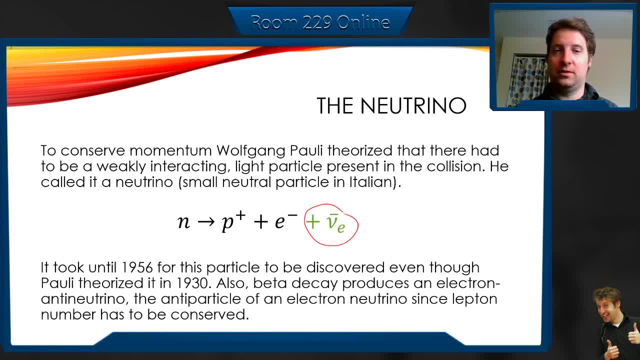 Which is Italian for small neutral particle, Neutrino. It's neutral and it's very small, Small as in very, very small mass. Okay, And it took until 1990.. 1956- so this was theorized in the 30s- took for 1956, actually discover where this, this particle. 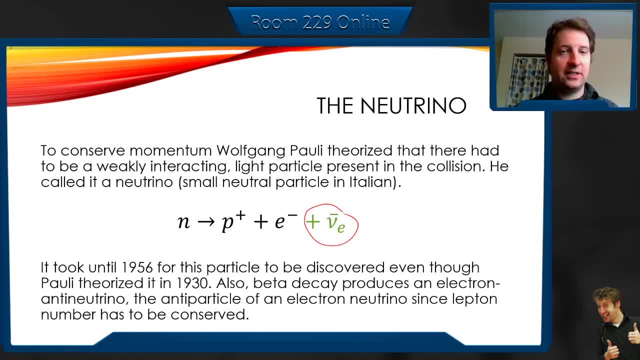 truly existed. that's because weak interactions are very, very difficult to to see because they don't interact with charge. we can't manipulate them- magnetic fields or electric fields, right? they don't. they hardly interact gravitationally, so we can't, we can't sort of weigh them right. so 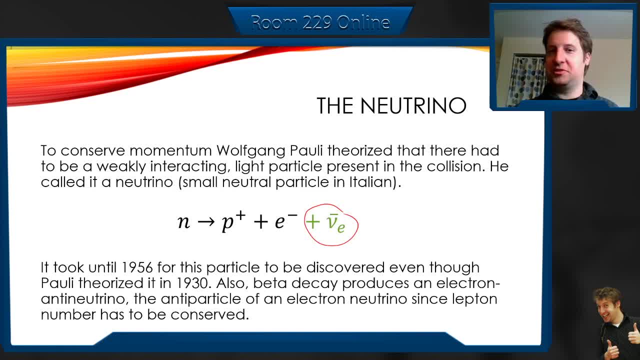 this has to, so we have to produce this. this third thing that's very, very hard to find now. what's interesting here also is this bar on top. this bar on top means that when I do, when I'm doing this, that bar on top to exist there. that's an anti neutrino. I have a regular neutron showing. 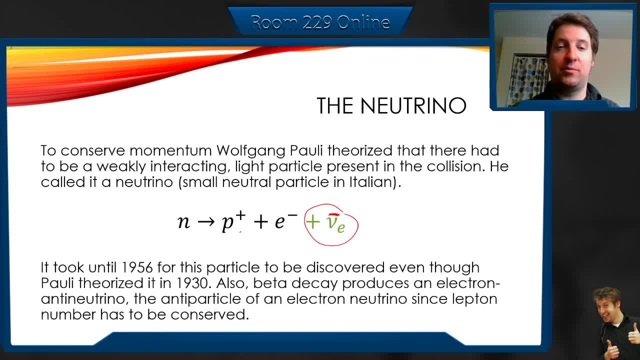 up here positron- I'm sorry, proton showing up here- and an electron. this is all regular matter, but I'm starting out with one piece of normal matter. two pieces of normal matter are made out of it. so to balance that, we call the the conserve, the lepton number- we have to have this anti particle show up. 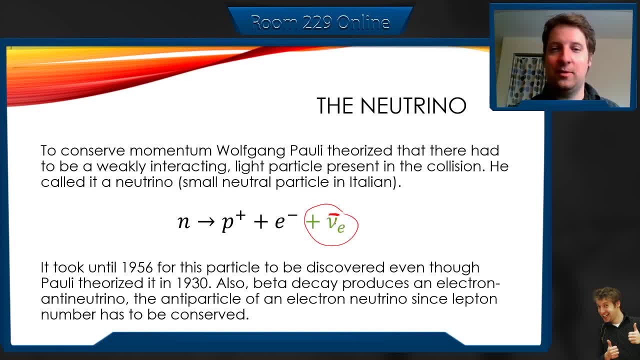 yes, this is a electron neutrino. I remember that's new. it's the Greek letter you and it's an electron. the flavor of a neutrino is an electron and it's an anti. this is an anti electron neutrino that shows up and that's because, when they call, lepton number has to be consumed. don't. 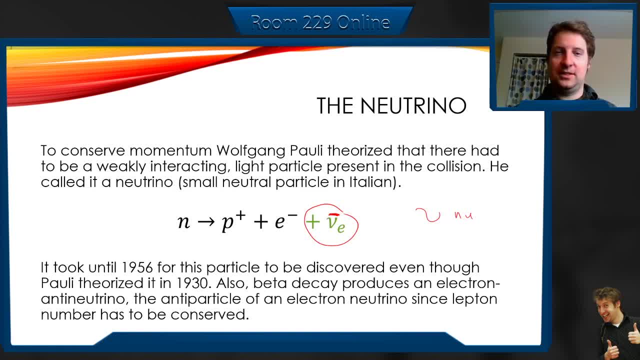 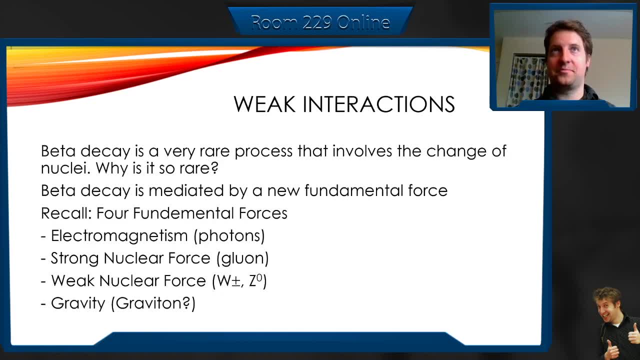 write too much, okay. so this is. this is the the modern view of beta minus decay. so these, this is a different view of beta minus decay. so this is the modern view of beta minus decay. so this is the our first example here of a weak interaction, and it's very hard to see and it doesn't happen too. 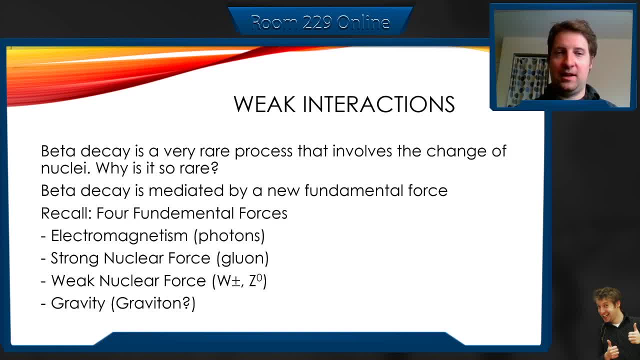 often because it's it's what we call a weak interaction, but it's moderated by the weak nuclear force. remember, if we go back, we have our, our fundamental forces, our electromagnetism, strong with nuclear force. so that's the force that holds the nucleus together and the weak nuclear force. 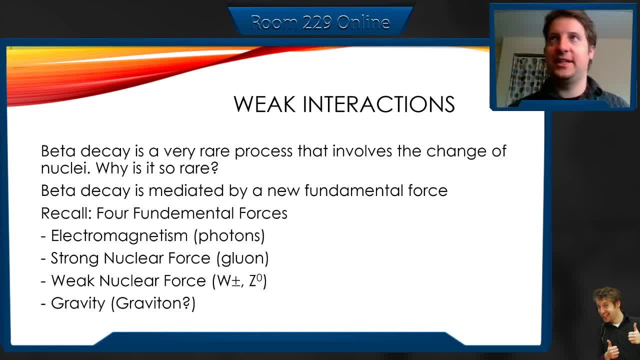 and then there's gravity you don't really understand. yet gravity does not fit into our standard model. where that's? that's like the? the holy grail of particle physics is: where is gravity in the standard model? we're not there yet. one day, one of you might discover one, okay, but people so? 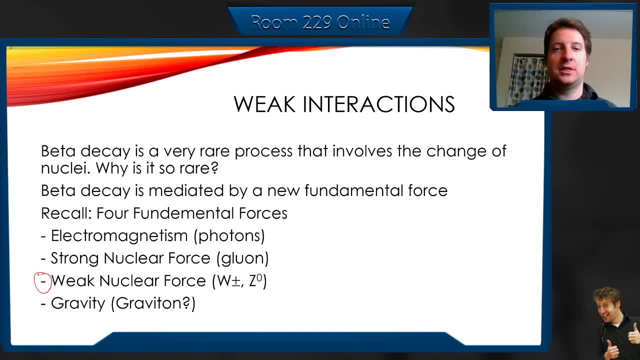 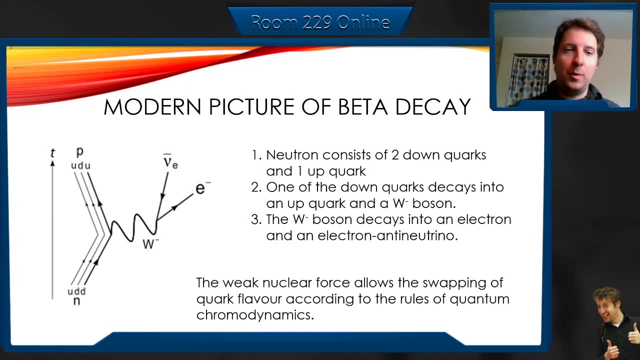 this, this one that we're talking about here, is called the weak nuclear force. that's moderated by positive straight W plus or W minus and or Z, naught boson, okay, and in our modern view, this is what happens. this is the, so what we call a Feynman diagram. there's a guy called Richard Feynman, probably, in my humble opinion, the most 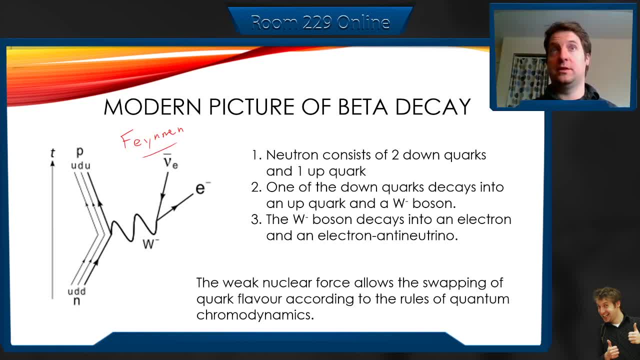 brilliant physicist of the 20th century- a century Einstein's up there. but I think the the fundamental work that that Feynman did in in understanding particle physics and just this fundamental view of the universe. brilliant man, Richard P Feynman, from Long Island, New York. he has the marvelous books. he had a. 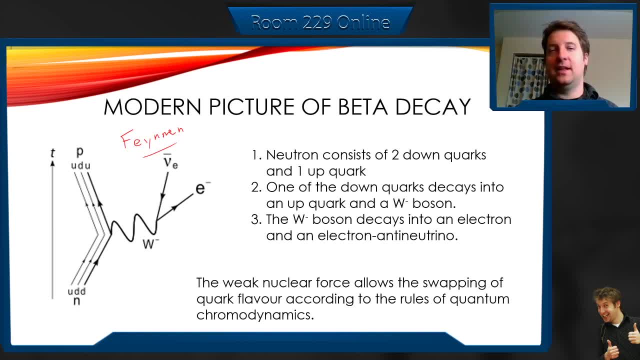 lecture series when he worked at MIT- oh sorry, Caltech. he was a lecturer at Caltech, did a course and then the course of books. Feynman lectures. there's three books I have a copy of them in. Mr Francis has a copy of them. they are the greatest physics textbooks. they're incredibly difficult to. 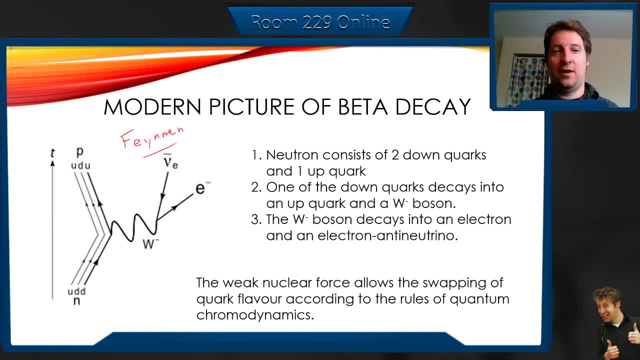 get through, but they are the best physics textbooks to give you an understanding of modern physics as it stands here. so what happens? this is a Feynman diagram. this shows a neutron here. this is where we start. okay, we have a neutron and it's going along and it's made up. 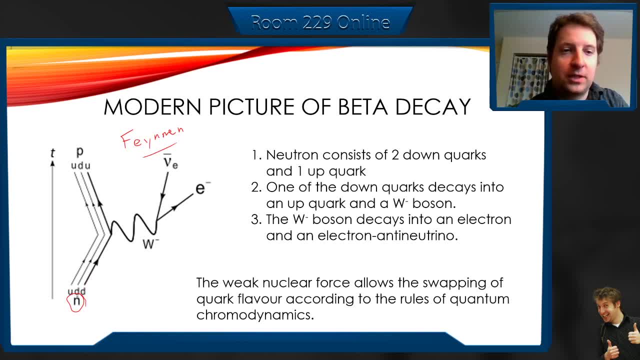 of neutrons are made up of quarks, three quarks: up, down and the down core. those are the. those are the quarks that make up a neutron, okay, but we have these these up, down, down quarks, okay, and this one down core comes along and at this moment it breaks down, it falls apart into an up quark. so this neutron is up, down, down. 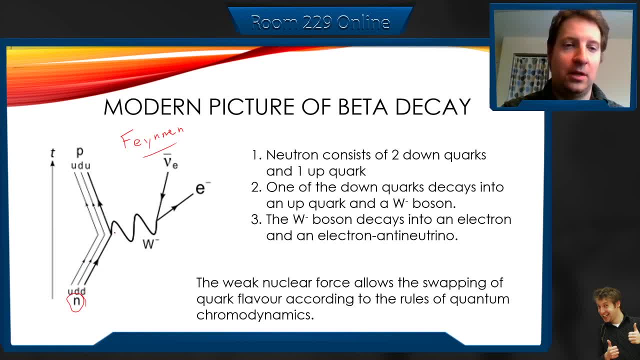 that made a neutron. one of the down quarks came along and at this point decayed into an up quark and at this point it was broken down and it fell apart and it's all over the place. and this is the quark. It changed its. it's what we call flavor. It changed its quark flavor from a down to an up. 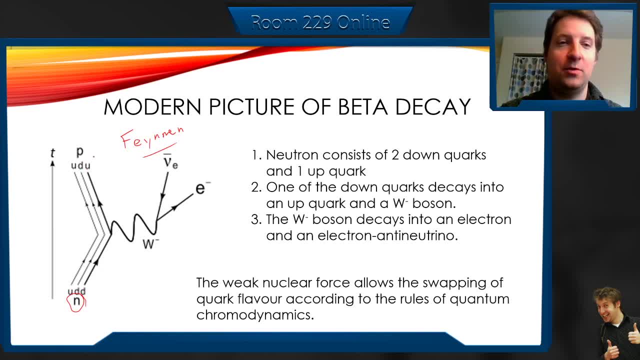 quark, And now we have an up, up and a down quark, which makes a proton, okay. So we went from a neutron to a proton, okay. So then what happened? also, for that to happen, it has to give off. 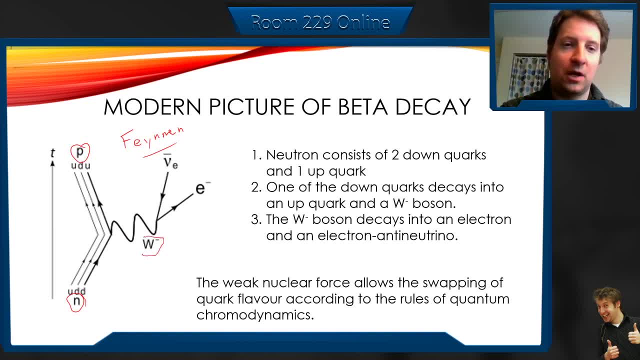 a boson right, Because there's something. some forces acted on this to change the flavor. It gave off this weak boson, this weak W minus boson. okay, So that's where that negative charge went to, because this went from a neutral neutron to a positive right To conserve charge. 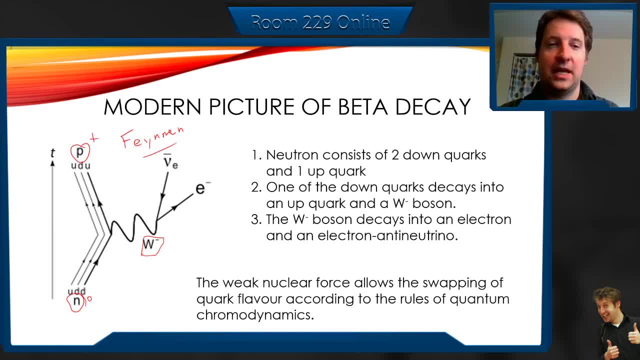 we have to have a neutral, a negative thing being. So that's a negative W boson. It exists as a virtual particle very quickly and then it also falls apart. We have that decay here, and this thing also decays into an electron that heads. 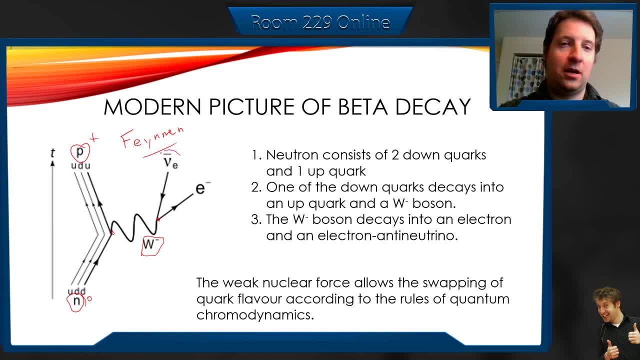 off this way. So there's our negative charge and our anti-neutrino, anti-electron neutrino, right. So first we have our neutron and then we have our proton. It decayed so that up down quark decayed into a boson and then the boson itself decays. 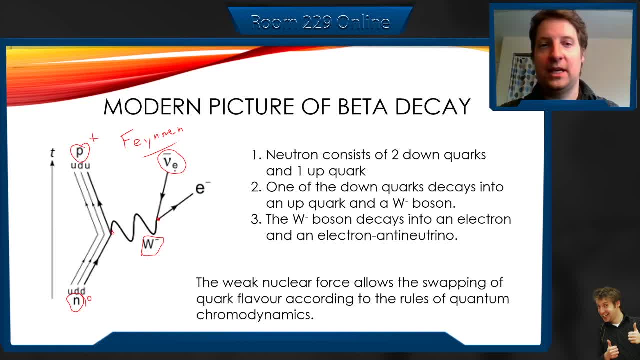 into a neutron, So that's a negative W boson Into two actual particles, which is an electron, a anti-neutrino. Now these arrows represent time. So time is going up. This x-axis doesn't really exist. It's sort of like a space axis. It sort 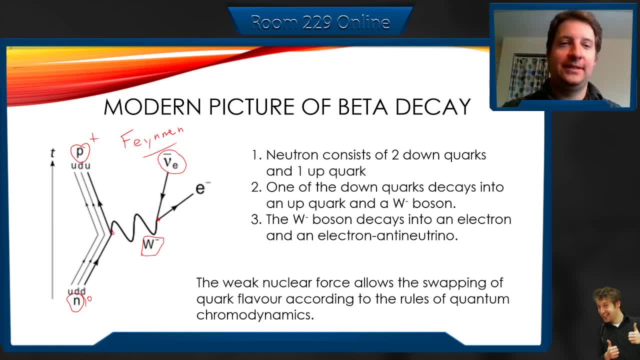 of gives us a sense of where this is happening. Notice that this arrow is down, which means antiparticles, from a Feynman diagram point of view, are traveling backwards in time. Really weird, And we're not going to think about that. okay, We're just going to leave that. 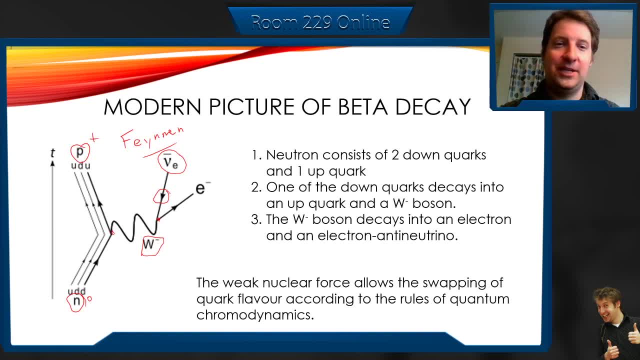 But the important point here is that this weak interaction, what it does is: it changes flavors of quark and it follows the rules of what we call quantum chromodynamics, QCD, which is a field of physics which we really don't understand. This is one of the frontiers of physics: quantum. 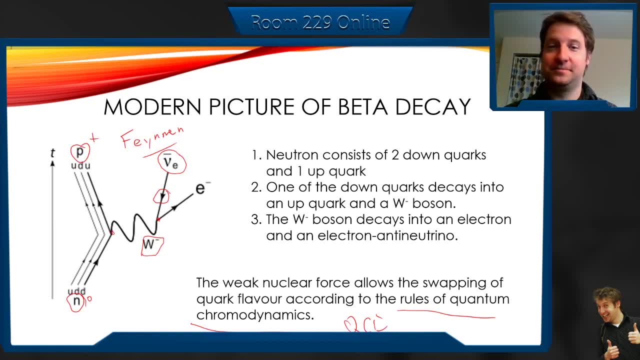 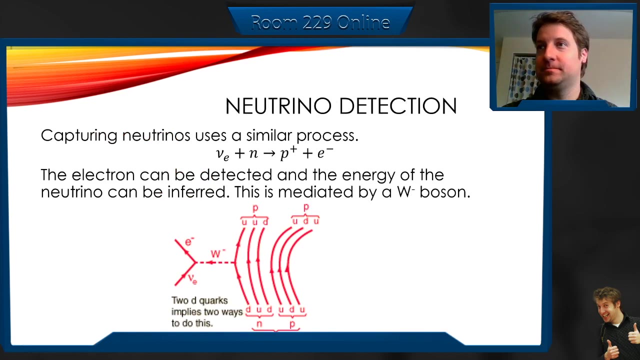 chromodynamics. This is the modern viewpoint of beta decay, right? So this is a neutron decaying into a proton, giving off two extra things, one being an anti-neutrino, the other one being an electron. okay, So the question becomes: how do we detect these neutrinos? Now, this: 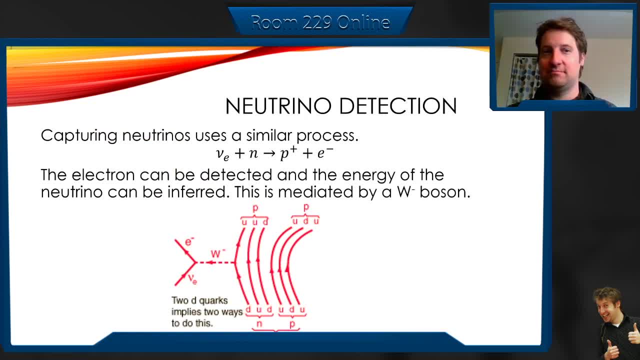 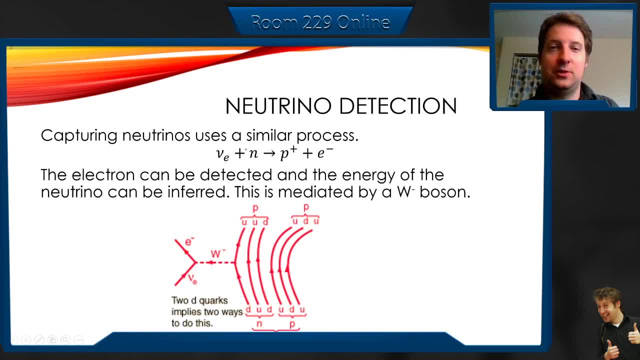 a neutrino coming along, electron neutrino come along and it smacks into a neutron. Oops, why? okay, Smacks into a neutron, Okay, And that creates a, a new proton and an electron, Okay, And this happens because we can see. 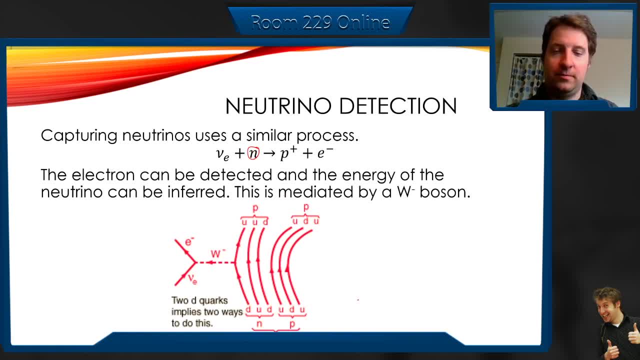 this occurring here. in these detectors We have a deuteron, which is just a hydrogen, regular old hydrogen nucleus, but there's an extra nucleus, So B is a thing Instead of hydrogen. hydrogen is a 1, 0. 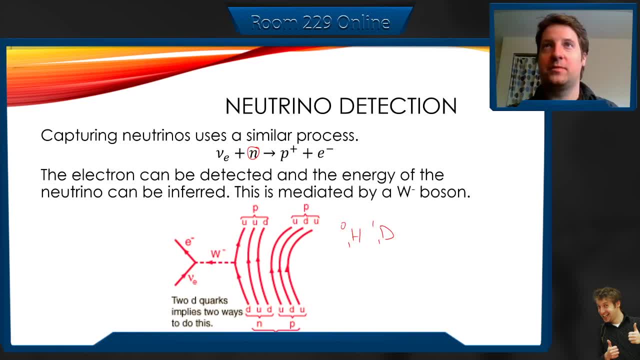 Deuterons are 1, 1.. They have a 1, 1. Hydrogen has a mass of 1.. Deuterons have a mass of 2, which means they have an extra neutron. If you put this into, let's say: take two deuterons. 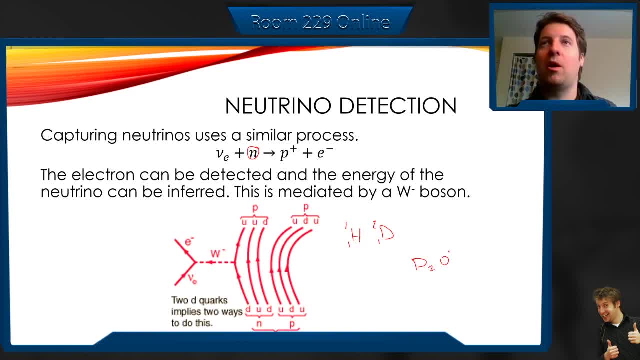 and add oxygen to it, you can end up with what we call heavy water. It's regular old water, but it has twice the mass. Well, the hydrogens have twice the mass, So each water molecule weighs 18 atomic mass units. 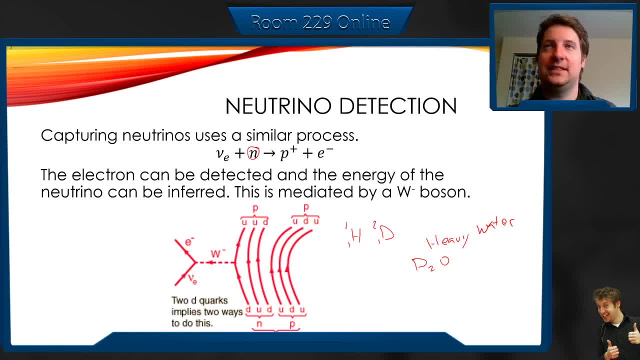 as opposed to 20, as opposed to 18.. So this electron comes with this neutron. The neutrino comes along And again, this is one of these Feynman diagrams- Takes one of the down quarks and transmogrifies it. 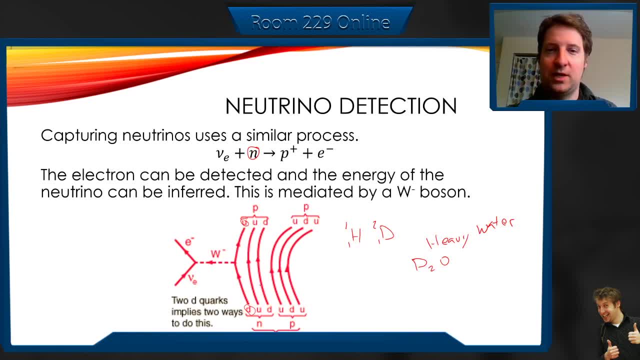 into an up quark, changing it from a neutron to a proton. So we end up having these two protons being created, the original one and the other one here, And we have an electron also showing up. So the input was a neutron. 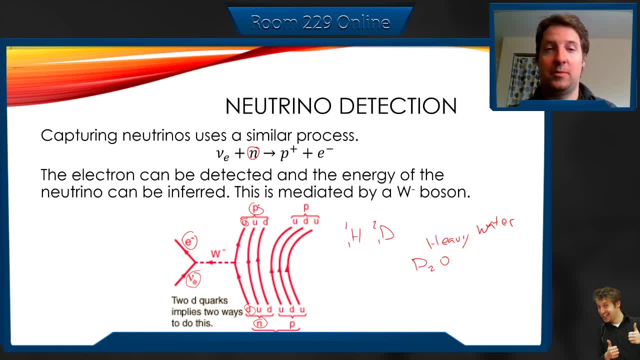 And a neutrino And we end up with a proton, and an electron come up. So we can actually see this. You take heavy water, you let it sit for long enough, you put a whole bunch of detectors around it and then you look to see electrons being formed. 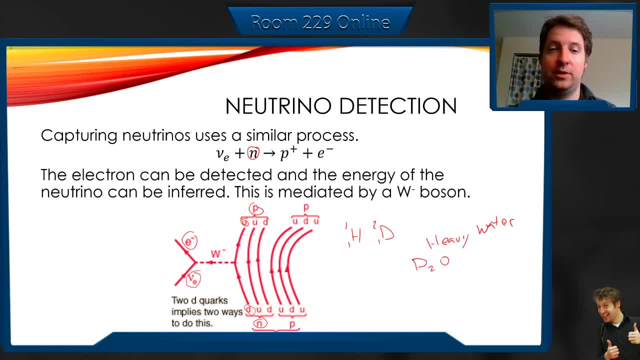 And this happens in our neutrino detectors, like the Sudbury neutrino detector or the one in Japan, or the ice cube down in Antarctica. That's what we want to see Another way. so that last one. sorry, this is mediated by a charged W minus boson. 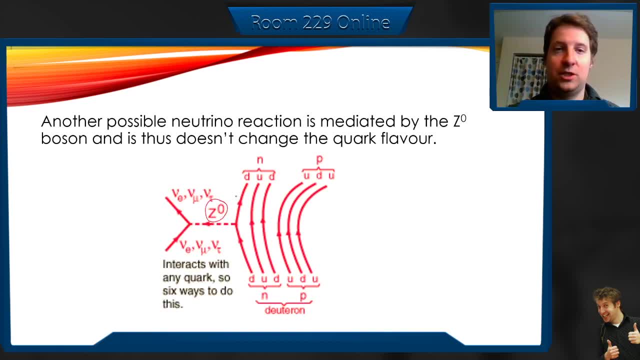 Or it can also be mediated by a neutral boson, which is when one of the neutrinos comes along and it just changes the flavor of this quark. It doesn't change the flavor, It can change the color, change the types of these. 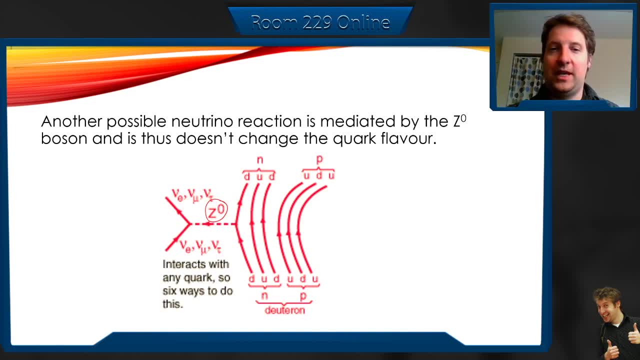 You've got it. This is very difficult to see. It's also another possible way of happening, but we can't actually see this in a detector. This is not a way. this is one of the other ways that happens. It's just not very useful for us from a physical point of view. 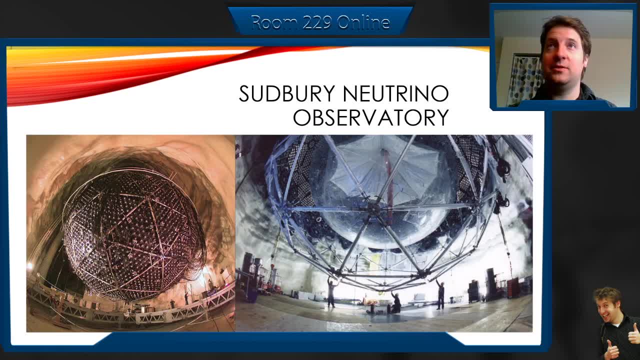 of detecting neutrinos. So here's the Sudbury neutrino observatory. So you can see in this picture, here, this big glass ball. it's an enormous glass ball and it's filled with that heavy water, It's filled with oopsie, it's filled with a whole bunch of it. 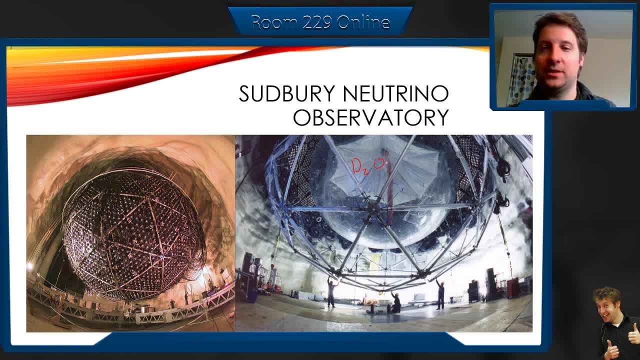 And then on the outside is all these detectors. These are called scintillators. They're electron catchers. basically, Sorry, not electron catchers. They're light photomultipliers. They're allowed to detect incredibly weak light sources. 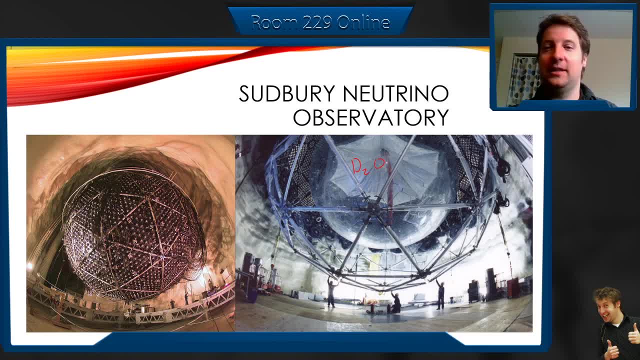 They multiply the regular light that comes in And then we turn it up into a much higher voltage and we're able to detect light. So this is it, with most of its detectors off. There's all of its detectors in here. This is the old Sudbury nickel mine. 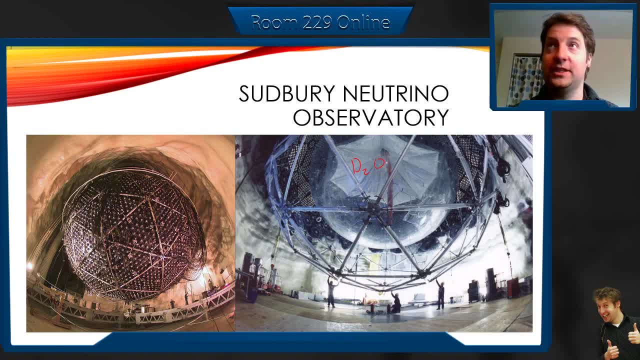 the big cavern in the old Sudbury nickel mine that they converted into the Sudbury neutrino observatory. So let this sit heavy water and they detect those electrons that come off. You've got to think to yourself: OK, so electrons are coming off. 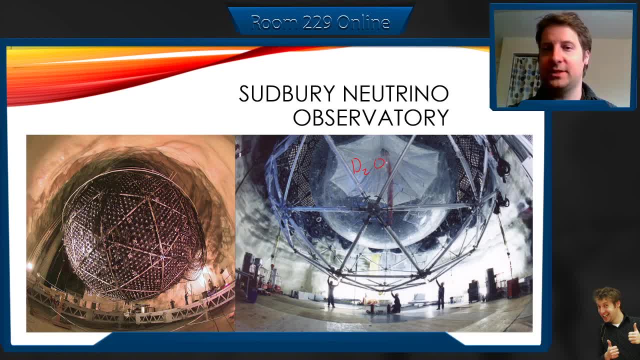 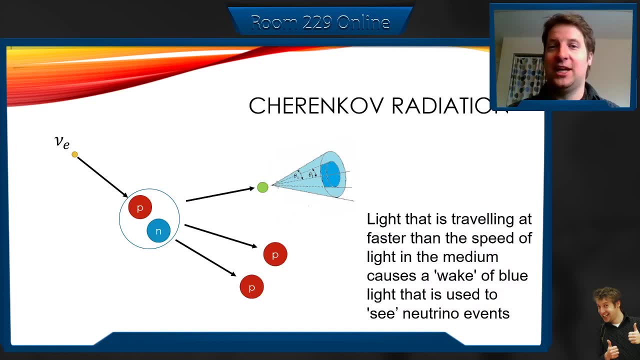 Why do we see light? Why is it important that these are photomultipliers that are detecting them? Where's the light coming from if these electrons are there? And that comes from this idea of what we'll call Cherenkov radiation. This is awesome. 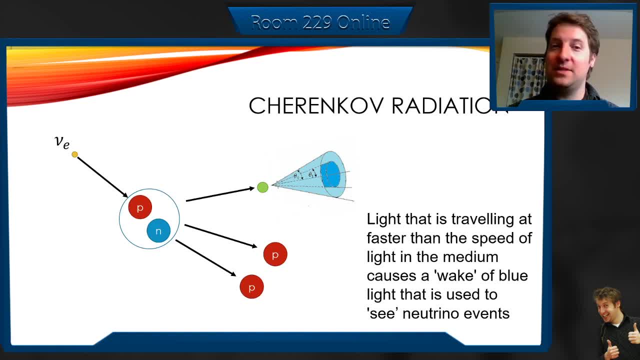 We always say that nothing can travel faster than light. But what happens if things do travel faster than light in their medium? So here again, this is our deuteron, here our heavy water deuteron, A neutrino comes along, smacks into the neutron. 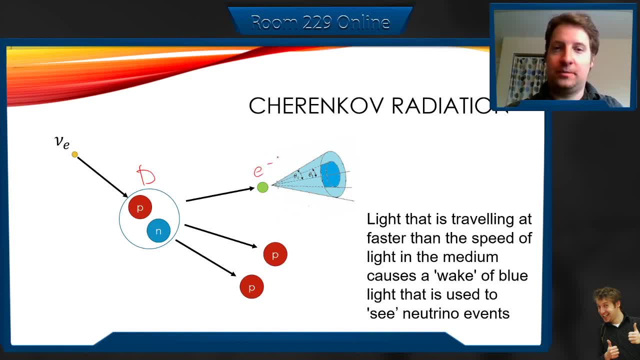 it creates two protons, and remember, this is an electron. Now, this electron has an enormous amount of energy and it's traveling very, very fast, And it travels faster than light. It's traveling faster than it should in the medium. 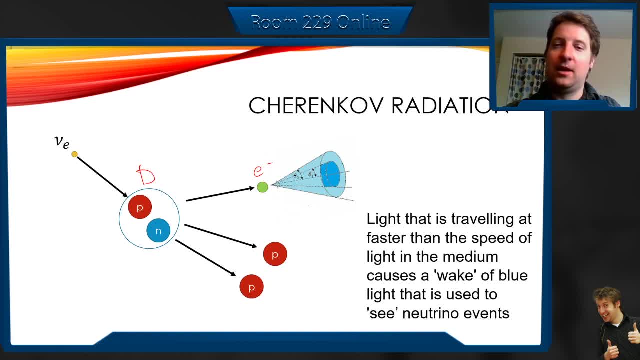 So when it's kind of it's a tricky idea here. So, OK, This is giving off light, because we know that light has a speed of c, which is 8.08 meters per second. Now remember, we learned in optics. 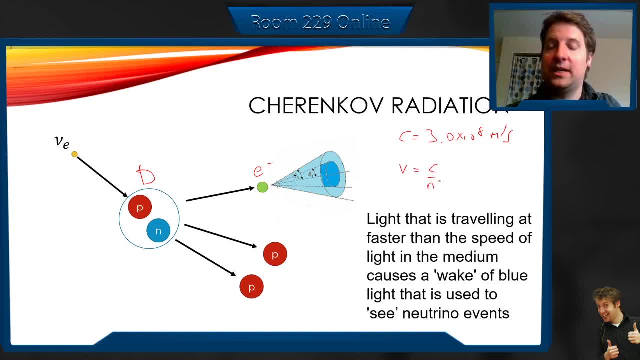 that v is equal to the speed of light in the medium divided by n, So probably the remember this is the index of a fraction of dense optically in a materialist. So heavy water is about the same as regular water. It's about 1.3, so 4 thirds. 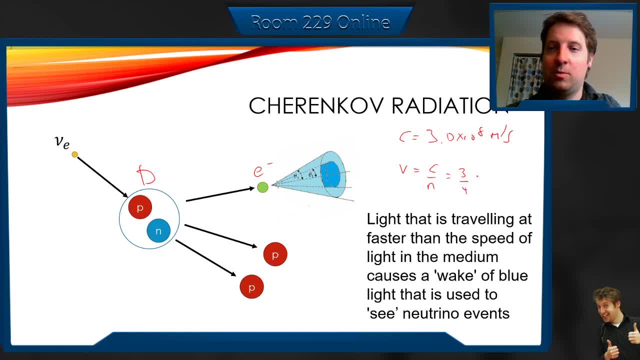 So this is going to multiply our c by 3 quarters. It's going to be 3 quarters of the speed of light. So if this electron is traveling faster than that, it produces what we call Cherenkov light. It produces this cone of blue light. 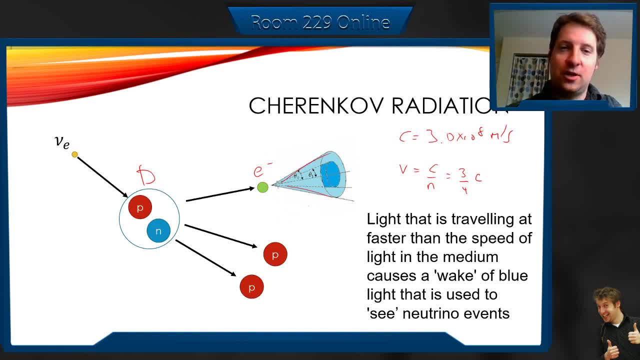 All right And it allows us to see that. So this electron whizzing at some ridiculous speed, because it's traveling faster, because it's traveling in this water, that has a speed of light of the speed of the medium, the speed of light in that medium. 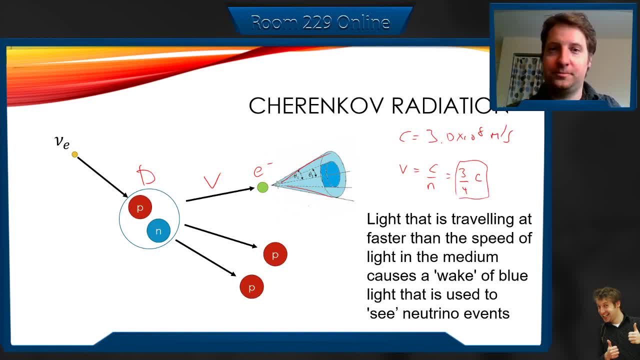 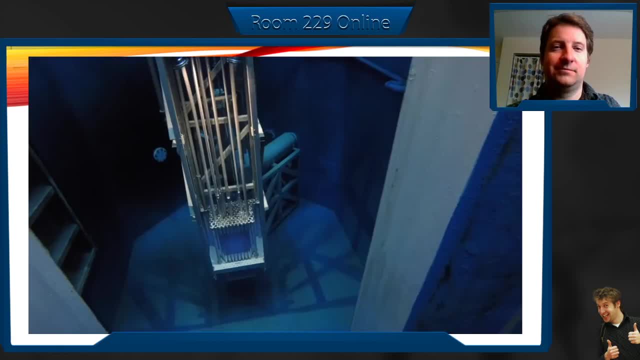 lower than the speed of light, it produces Cherenkov radiation. You may not believe me, but check this out. This is a nuclear reactor. It's a research reactor, but still a nuclear reactor. It's a whole bunch of uranium in there and they're going to turn it on. 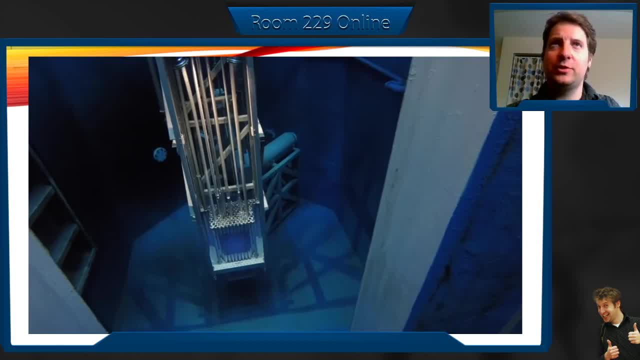 They're going to start the fission process, and the fission process produces all kinds of radiation, tons and tons of radiation, a immense flux of radiation. Let's see what happens when they turn it on, And this is immersed in water. 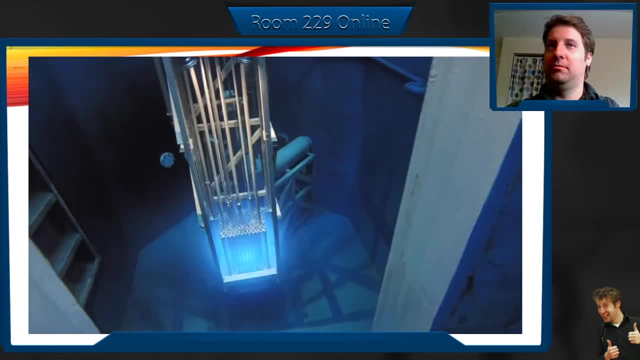 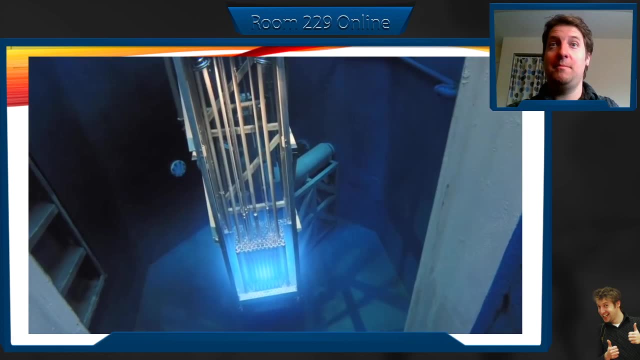 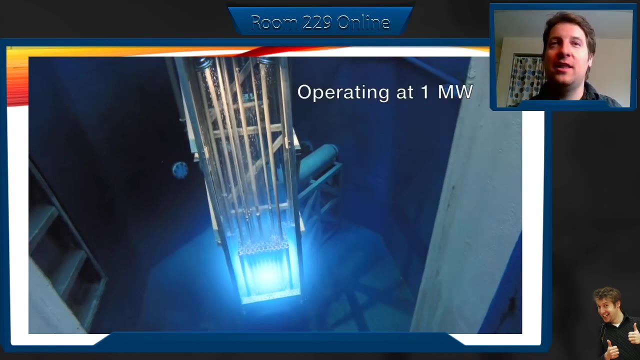 Watch what happens. Where's all that blue light coming from? Where's all that blue light coming from? That's Cherenkov light. That's all the decaying radiation. That's all the decaying radiation. That's all the decaying radiation. 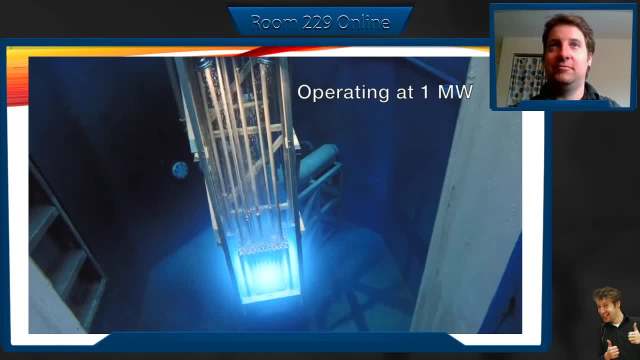 The decaying materials that are coming off of the uranium fuel rods in there, just glowing bright blue. We're totally safe here because that water is actually stopping all those radioactive particles from getting to us. If you were standing there in front of 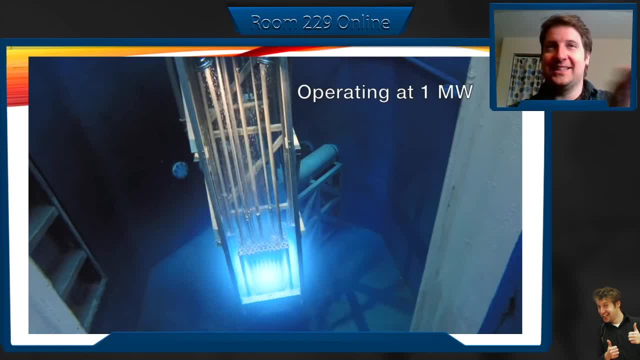 I don't know if that's glass or if that's a camera. It is a camera, I guess, because we can see it, but I don't know if you can actually observe this in real time from a glass window or something, but it wouldn't matter, because the water is stopping. 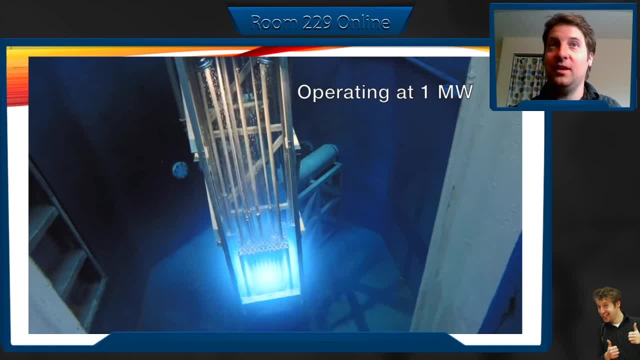 all the radiation you can see, that blue glow of all that Cherenkov light coming off of there. exact same thing happens in the submarine neutrino observatory, but it's it's uh, much, much, much weaker, and it only happens like once every two days or something, right? so this is Cherenkov light, this. 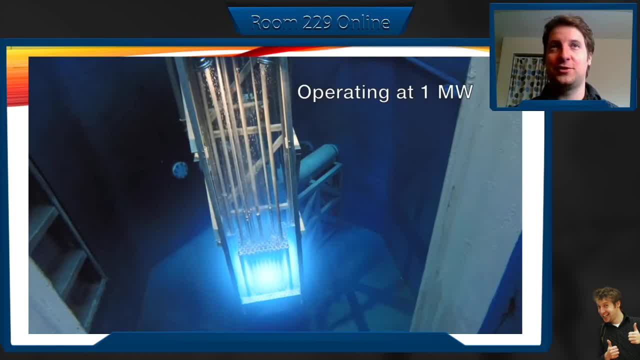 is a much more luminous version of Cherenkov light. the same thing happens in uh, the the um submarine neutrino detector. also happens at snow, which is the uh, the ice cube. sorry, snow is the submarine neutrino observatory. there's another one, called ice cube, in Antarctica. I'm gonna put. 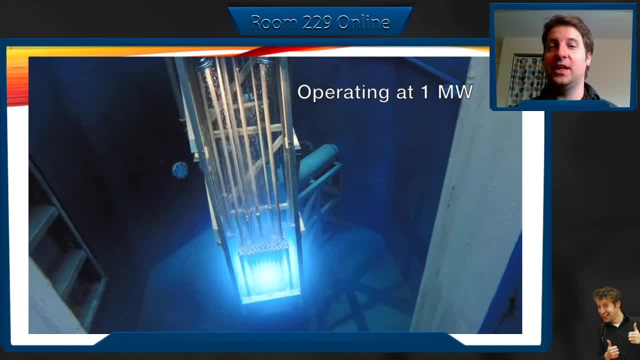 a link in the check, in the link in the in the description for this video of a bunch of different videos describing how this is done. one of them is called ice cube- how they built ice cube um, why neutrinos are cool. just check out all the videos, okay in there.